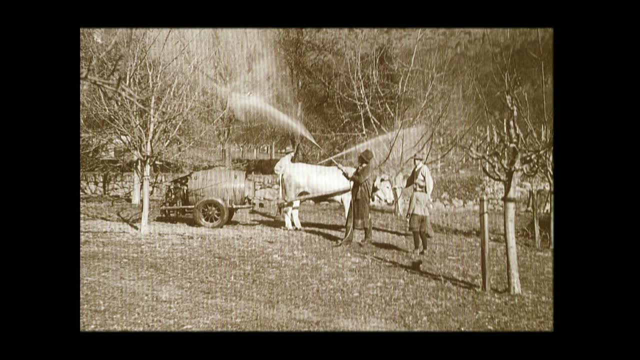 Part of the way the story gets told very often is that they They really amplified after World War II, And that is in fact the case. They did amplify because we were able to use so many of the different chemicals that were utilized in World War II, defoliants being one various insecticides. 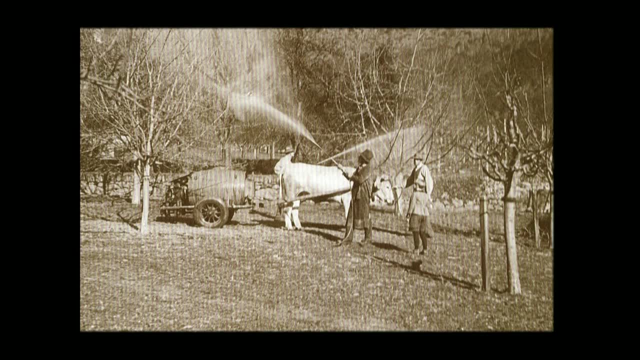 But they actually go further back And it's kind of an interesting thing when you look at fruit production and vineyards in particular, because what happened was in Europe they were very taken in the late 1700s, early 1800s, very taken by the different kinds of grapes that they found. 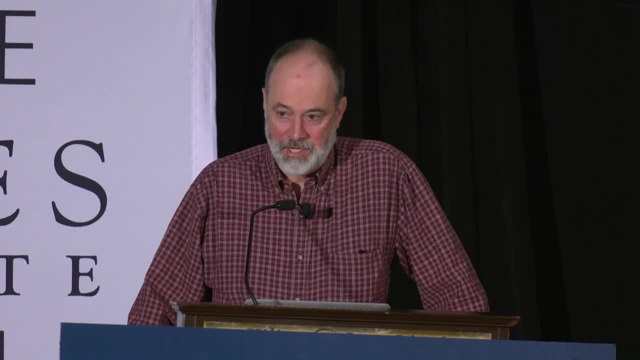 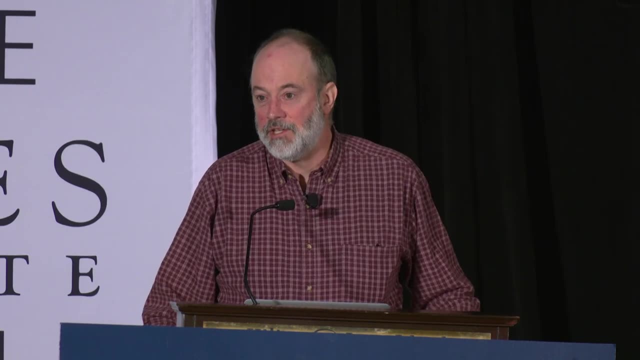 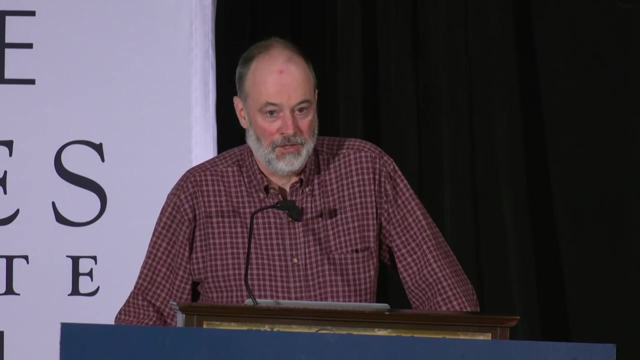 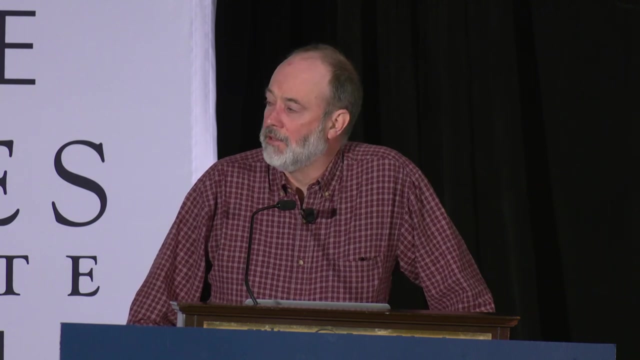 And the United States and the different tastes and the wines that they made, and Thomas Jefferson and others were very prominent in this whole move. So they actually took some of the vines from the United States. They took them to Europe And unknowingly, when they did that, they also took two fungal diseases and then also a louse, the rabe louse as it's called in German, or the vine lice- phylloxera is the Latin name for that. So they took those three things with them And it took a long time. It didn't take long for those two fungal diseases to spread and it didn't take long for the vine lice to spread, but it took a long time to figure out what was going on. So, finally, the Europeans started to realize that their vineyards were dying and they were getting hammered and they couldn't figure out what it was. Eventually, they figured out that there were the phylloxera, the vine lice, that were in the soil, that were underneath, that were killing them. 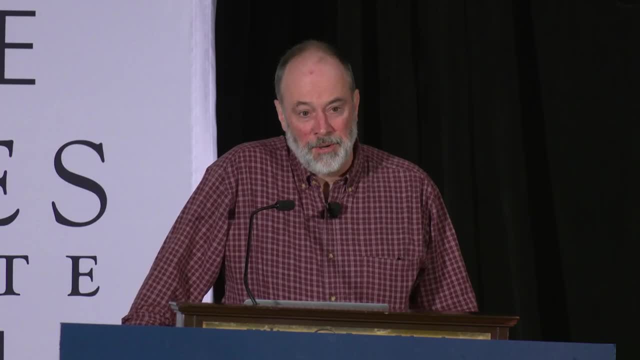 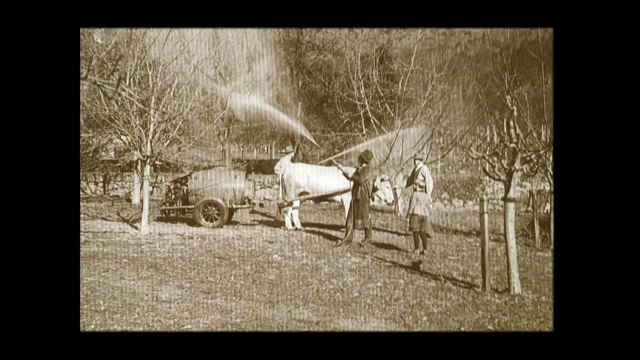 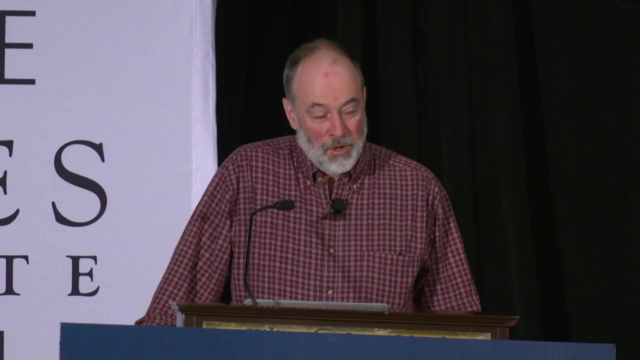 And they started to figure out the two primary diseases that the vines were having, the fungal diseases, And, as a result, they started with what you might, even these days here, refer to as the Bordeaux mixture, which is basically copper and sulfur. And so this mixture of copper and sulfur, that wasn't the first pesticide, necessarily, but it was one of the most widely used. 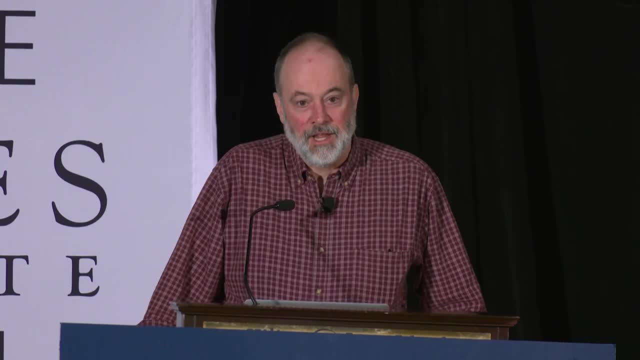 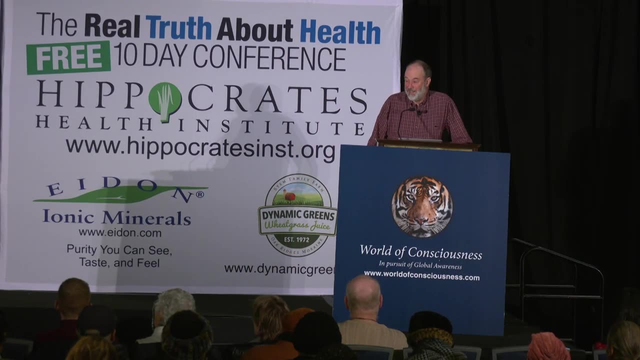 And so it was used in Europe. Then we also brought it back to the United States And, you know, fairly effective in some cases for some of the fungal diseases, but that's primarily what was sprayed. Unfortunately, at one point arsenic was also in the arsenal. 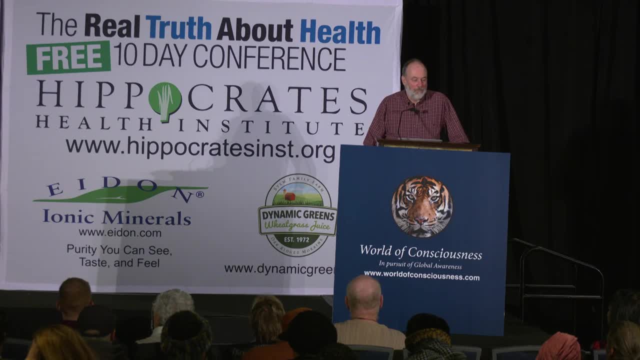 You know, Which is a little bit ironic. So pesticides have a long history And I should also say that when you look at cultures like India, there are pesticides there that are organic, that have been used for millennia, that are naturally occurring. 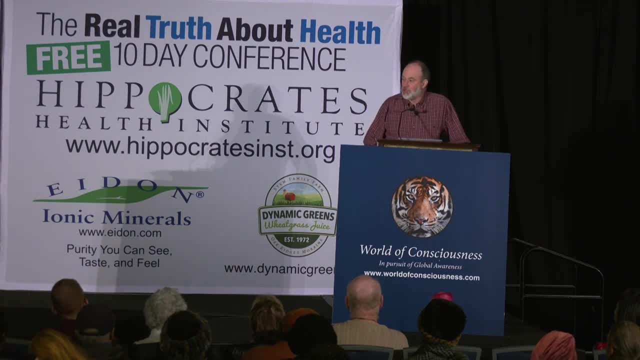 And so I think we need to remember that actually, these things have a much longer history than we generally talk about. And in this case, what they were spraying for I'm pretty sure this is probably a petroleum distillate, probably a white oil- Weisserl as it's called in German, and against the tree lice. 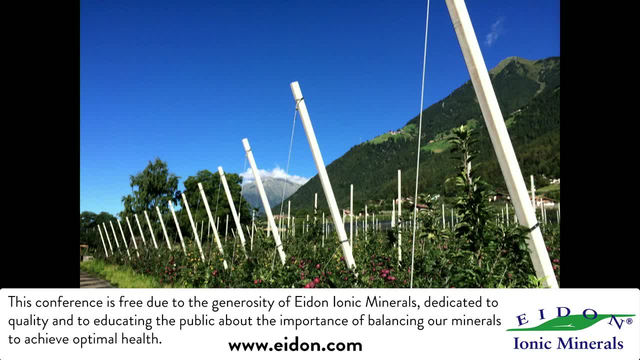 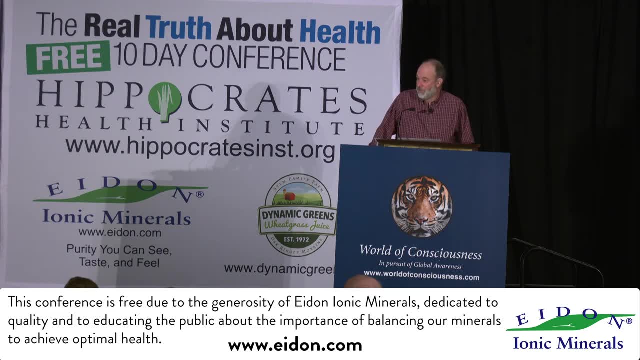 In that particular case. So the small village that I've been going to since 1983, it used to be a very diverse agricultural village. These days, as you walk around, this is almost all of what you see. These are the apples. 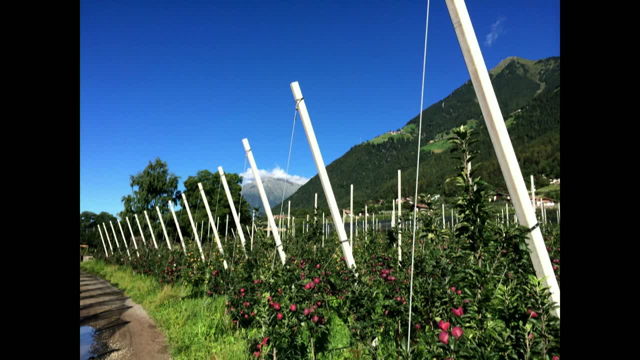 And we're here just outside of Big Apple- This is Big Apple in the Tirolean version- And you know it is just amazing what's happened in terms of the transition of the landscape, And obviously with that comes the use of a lot of pesticides. 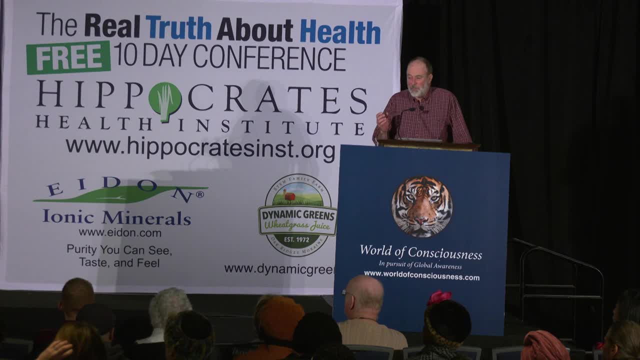 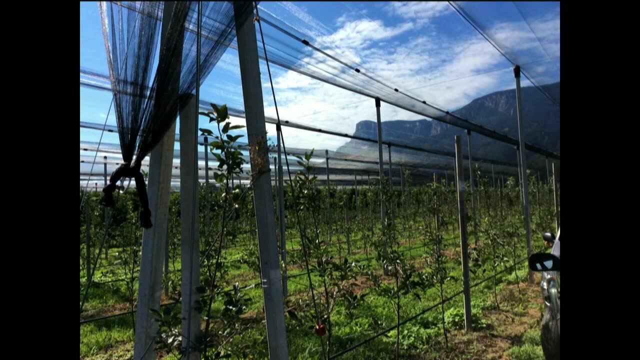 So this is what things look like. The Tiroleans- as I said, the cooperatives- were just incredibly smart as they were thinking about how can we actually really start to market apples, make a good profit for the farmers? And so one of the things that they discovered was in 1973, the Dutch were doing a really fantastic job with what they call the slender tree trellis system. 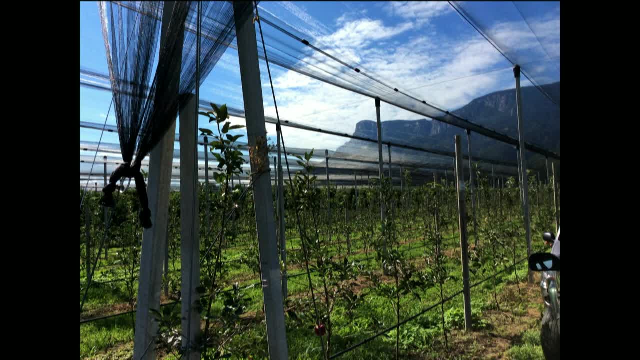 So that is, and you'll see this more and more in the United States. This is something that you start to see quite a bit, actually, in upper New York state, starting to see it in Vermont. Some certainly see in Washington state, And the idea here is that you try to grow the tree. 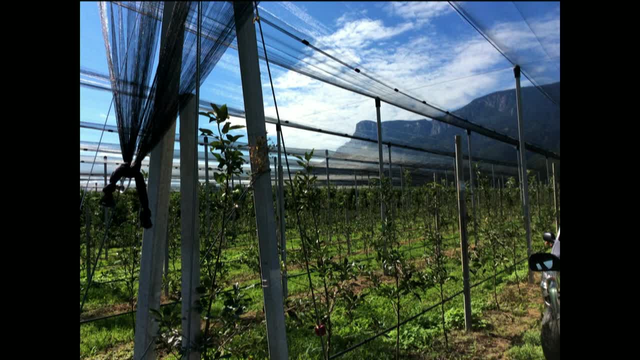 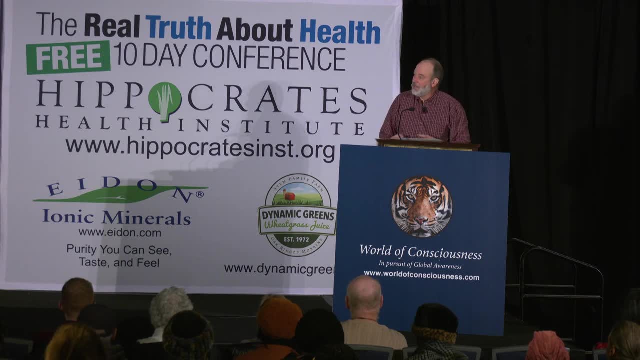 You use a dwarf or a semi dwarf rootstock So you actually keep it, so it's not going to be too high. It's when you're able to do this instead of having the full size or the standard trees it's actually of some benefit because you can do everything easier. 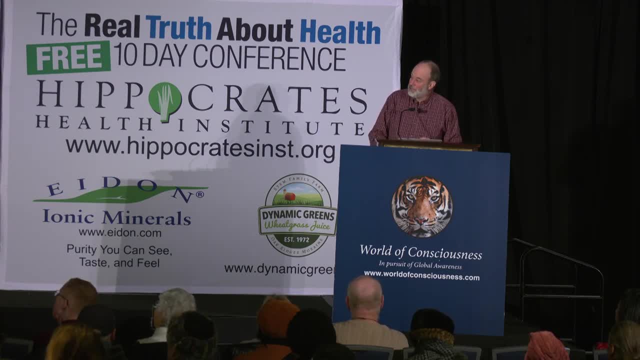 You can certainly do the pruning easier. It's easier To do the irrigation- as you can see here that set up- it's easier to do the spraying. in theory at least. what's touted is you use fewer pesticides because you're not having to spray into this really deep vegetation in order to try to penetrate to the middle of the tree. 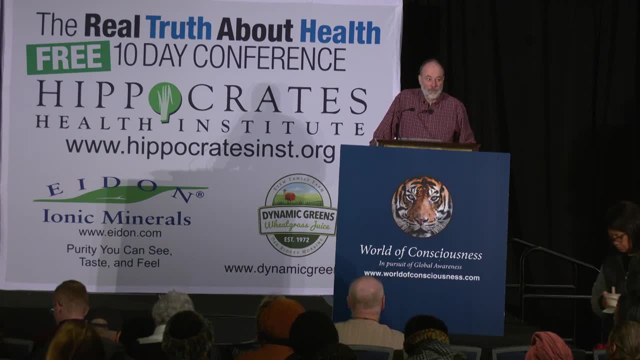 So there are some advantages to it, And certainly the harvest itself becomes somewhat easier. Part and parcel of that these days is also putting what you see here on top. These are the hail nets, and the hail nets are actually- I mean, they literally. They are an insurance, but they also mean that the farmers don't necessarily have to buy crop insurance. Instead, they invest in these hail nets. So the hail nets protect against a very volatile climate that you have there, especially with climate change right now in the Alps.